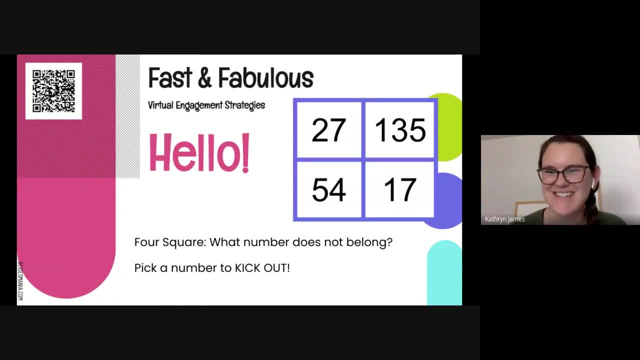 one Send everybody. Which number should we kick out? Interesting? So this strategy- four square- elicits responses from students and, as you can see, everyone has very, very different responses to which number they wanna kick out. I think almost every number was chosen. 27 was not chosen at all. 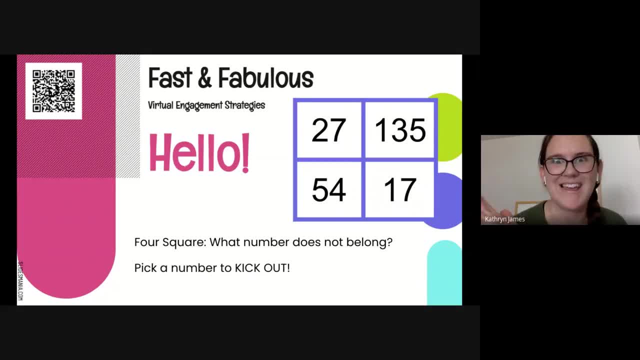 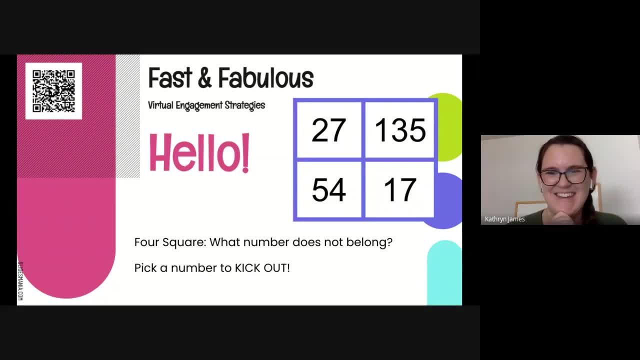 I chose five this fine afternoon. I chose 17 because it's a prime number. 17 because it's a prime number. Does anyone agree or disagree with that response? 17 should be kicked out because it's a prime number. I see Jennifer Johnson said 135 because it is a three-digit number. 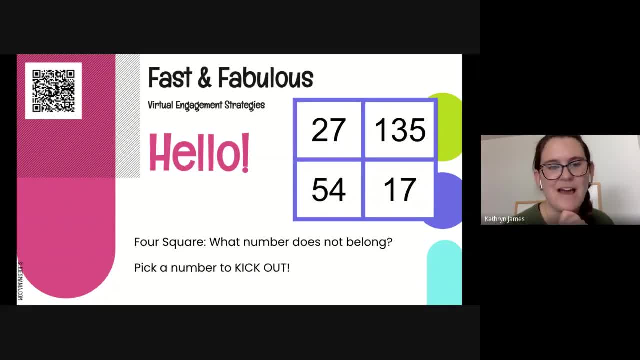 Andrea, you also said 135.. Do you have the same reasoning or different reasoning? The same, And, Jenny, do you agree or disagree? The same, And 54 was up here a couple times. Does anyone want to say why 54 is the number that does not belong in this fourth square? 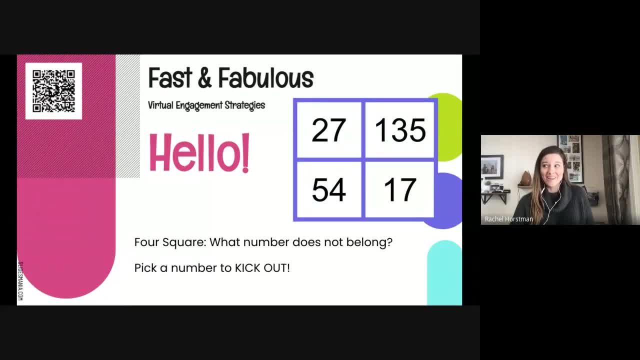 I chose 54 because it is the only even number. Beautiful Thank you, Tricia. So I'm going to point out a couple of things that maybe, in this fourth square, might get your students to think more, depending on their grade level. but which of these numbers is not a multiple of nine? 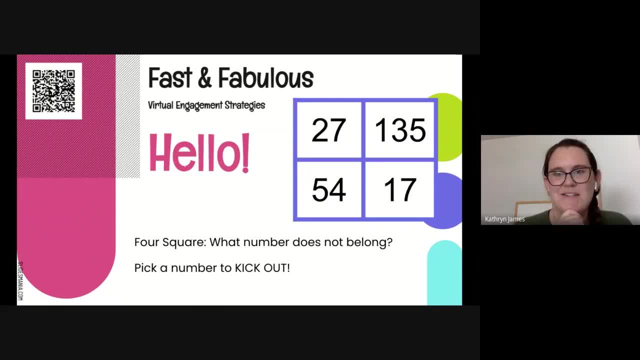 Is there another reason to kick out a number If you add up the digits to these numbers? is there a number, when you add up the digits, that you might want to kick out? So this activity four square lends itself to rich discussions on mathematics, where every 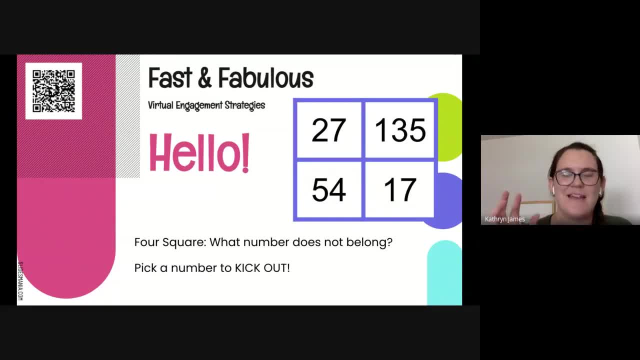 answer is a correct answer And it's a beautiful engagement strategy. And it's a beautiful engagement strategy. And it's a beautiful engagement strategy because it means every student's opinion is like valid and they get to engage right away. with what number do you want to kick out? So welcome to Fast and Fabulous. We care about engagement. 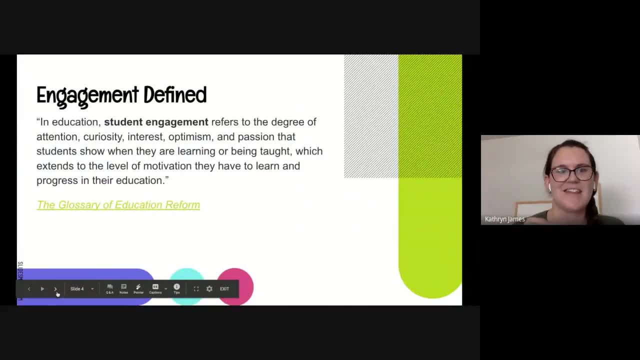 because it is the root of our students' joy in learning. It speaks to their attention, their curiosity, their optimism and passion in learning. So when we're talking about engagement, we're not just talking about camera on, but in a practical sense it does mean our students are. 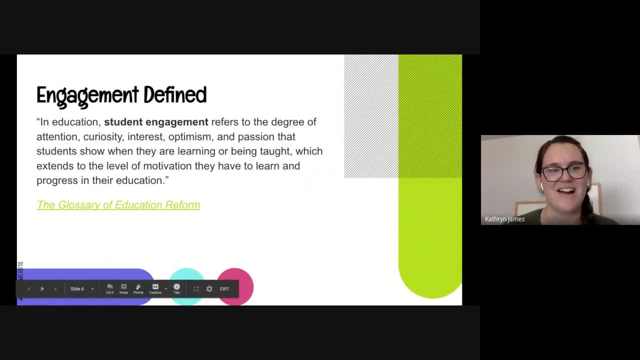 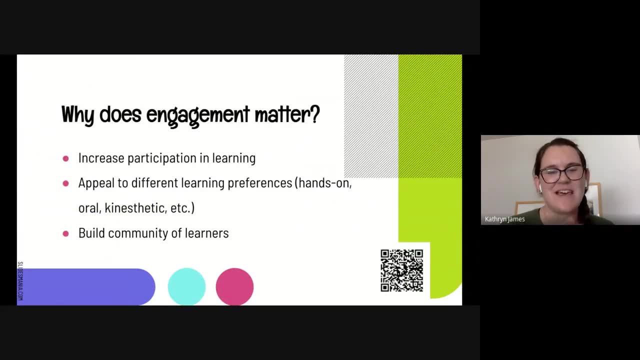 participating more. We do see that our students are engaged in the ways that we can quantify and observe. And on the next slide, Rachel, we have a couple other things that might appeal to you as a teacher, like why engagement matters. It's appealing to those different learning styles. 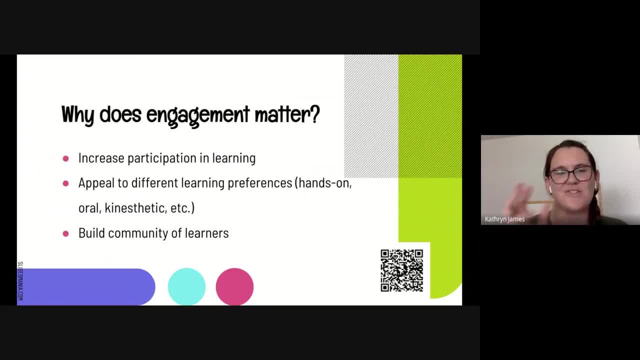 and it's building a community of learners, Like this fourth square activity. if your students are used to this as an engaging activity, they will see that this is a community of learning where my opinions are valid and I have an opportunity to express them in multiple formats. 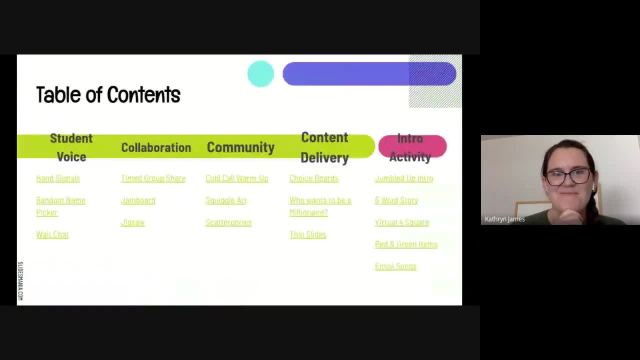 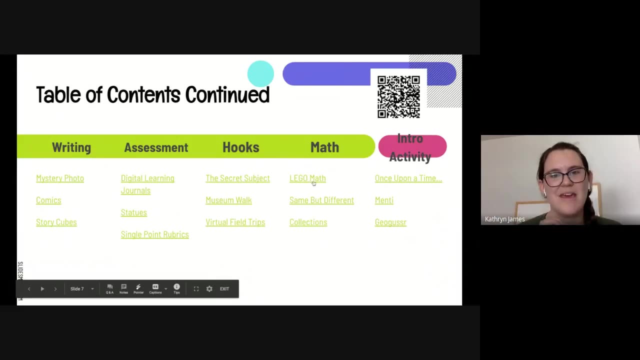 not just through the chat box, but also in dialogue. So this is Fast and Fabulous. It is a ton of strategy. We're going to be looking specifically at math strategies for the very first time And we have three for you. We have Lego math- same but different in collections. And Rachel, will you click on? 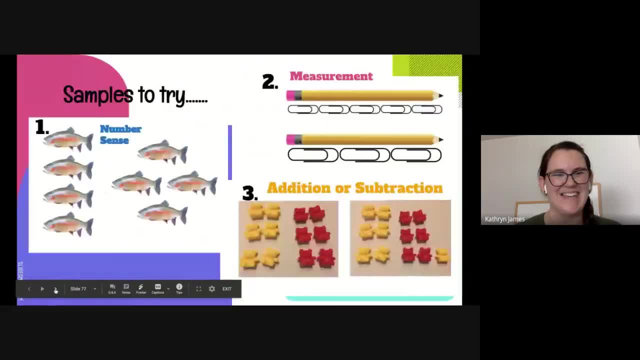 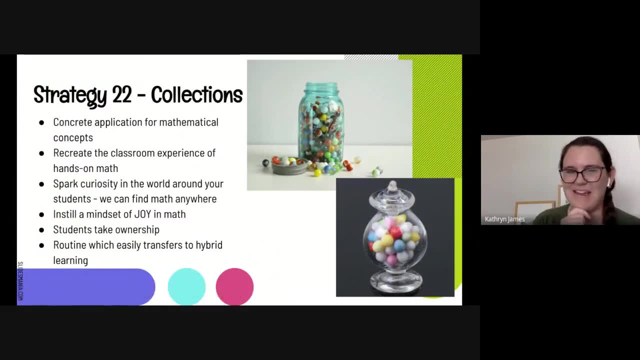 collections for me. Thank you One more. So our first engagement engaging activity for math is collections. So when we are facing the computer with our students, there's a lot of virtual, and so collections is a way to engage with your students in the world that's around them And I 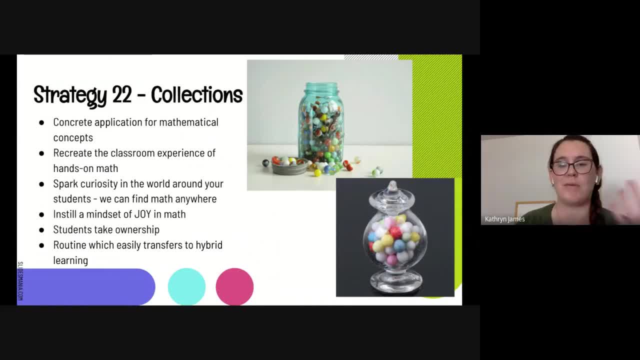 would encourage this as a strategy, used once or once a week, maybe once every two weeks, But just literally going through your environment and filling a glass container with a collection. In this case, I have different kinds of batteries and I might even pull them out and show how. 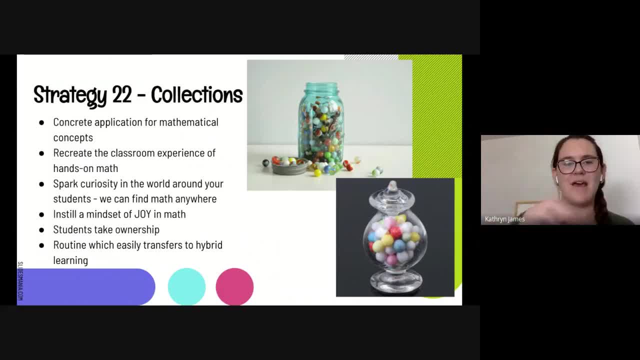 they're different sizes because that will help with students estimating. But in this we are creating a concrete application for a mathematical concept which can be estimating the size of the building. It can be multiplying depending on the targeted skill. So we're going to recreate a 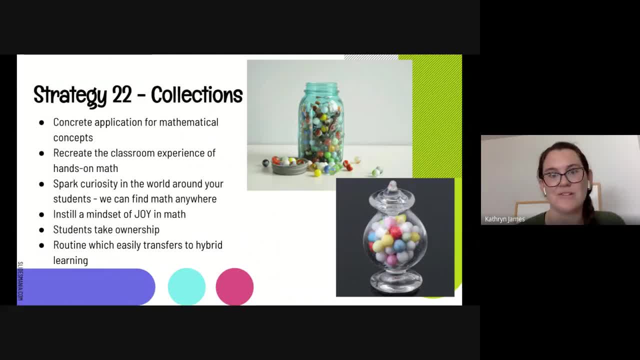 classroom experience. You definitely have done this before in your real-world classroom, which is giving a collection to students and having them first guess how much they are and then tallying or counting and actually finding the actual amount. This can spark curiosity for your students in the 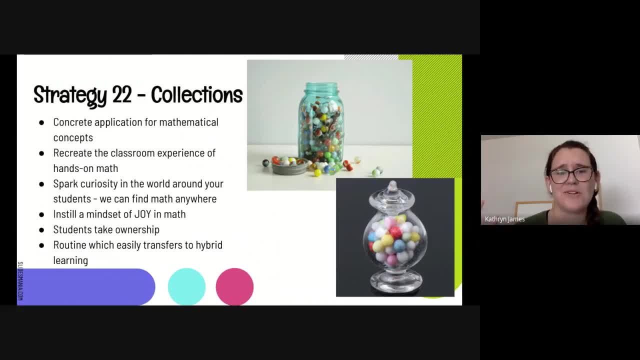 world around them as they go about their world. If I'm in the grocery store, I might guess how many pieces of spaghetti are in a package of spaghetti. I might guess how many pieces of pasta. But it instills this mindset of joy in that, because you're really giving students a way. 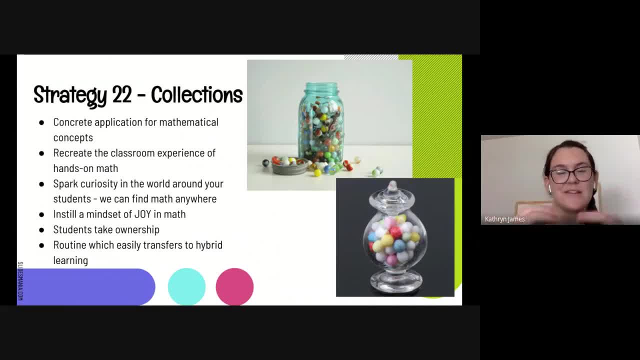 to apply a concept that's hands-on and the items themselves can spark curiosity, And it gives students the opportunity to take ownership. And this routine will easily transfer to hybrid learning, which is another great plus for this particular strategy. Here I have batteries and 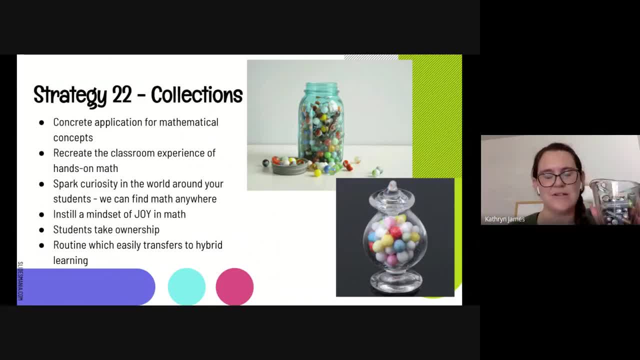 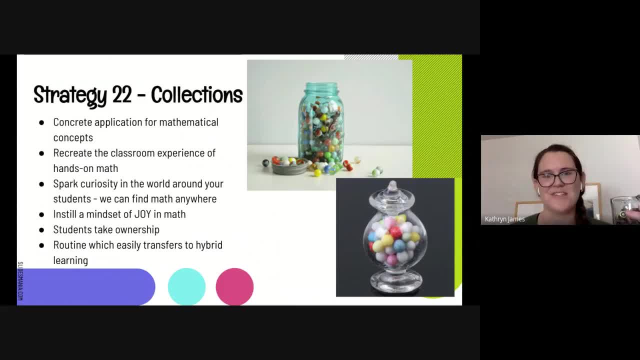 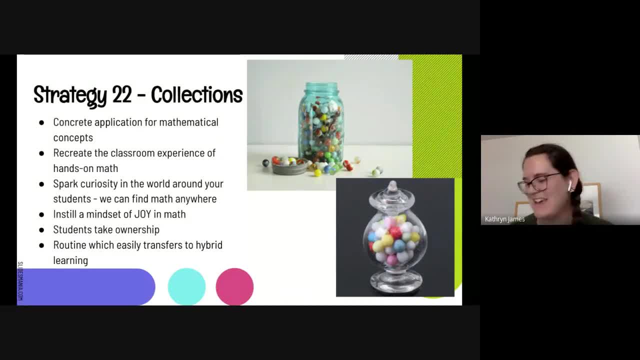 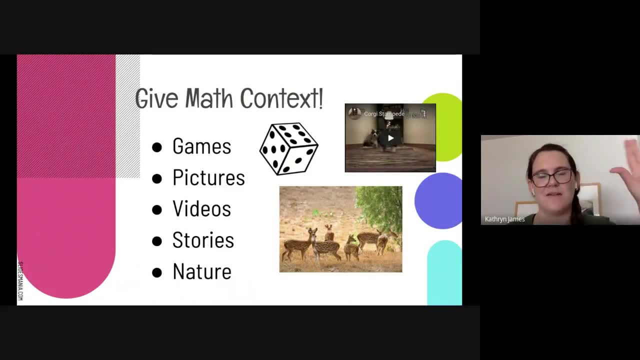 you're using, or using like a glass jar, like you see in these pictures And on the next slide. thank you, Rachel. I have some other ideas for giving your math context: just taking something that is theoretical and applying it to a way your students can engage a little bit more, And so. 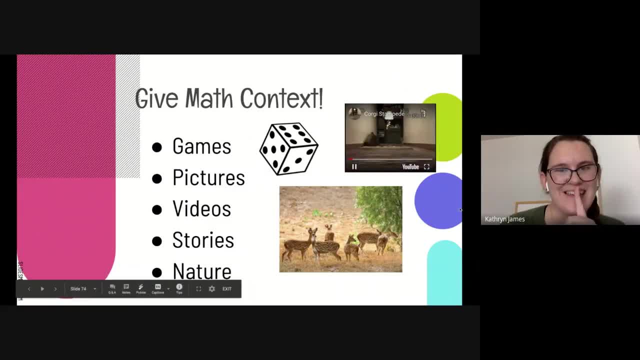 would you play that video for me, Rachel? But right before go ahead, How many puppies did you see? Were you able to sympathize? That's one of my all-time favorite videos on the internet. It's very old, you can tell, But it just evokes for me a great way for 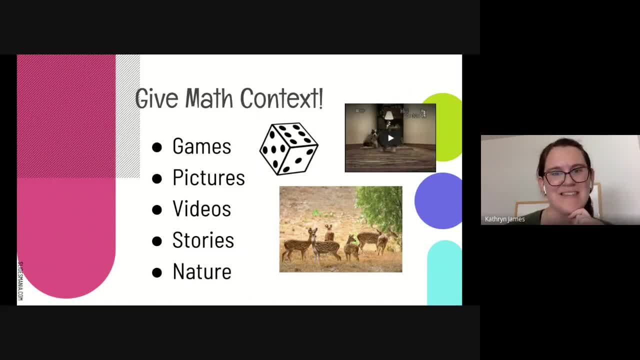 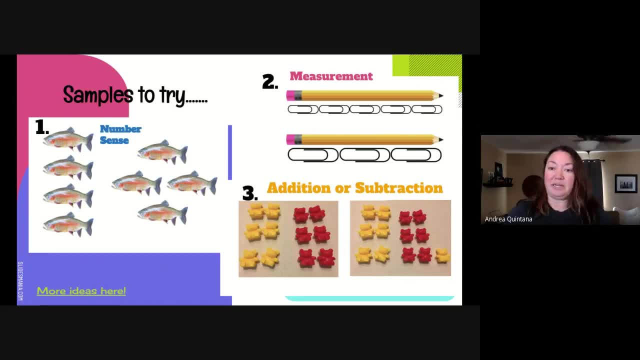 of course, I have a picture here looking at the real world, looking for wildlife, And then come up with- And there might be a million different answers And there might be just a couple that you can build off of with those talk moves. Now I shared a website where I got these: 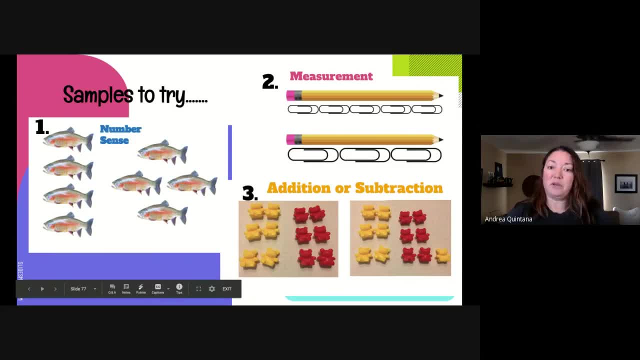 images from here- It's clickable in the slides for you- where it goes from everything from number sense, which is the basic foundation of counting, It goes all the way up to algebraic thinking. So if you have students that really need to be pushed and enriched, you can provide them examples of 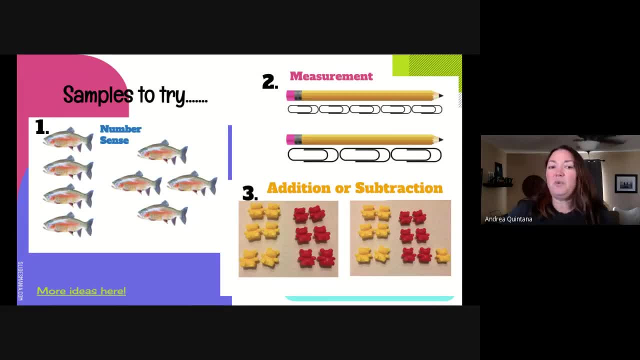 this that really meet their need. And so let's try with number two, which was kind of in the middle of these two objects right here. So, for measurement, try and write a sentence in the chat Or, if you're brave, you can unmute yourself and share your answer. I'm going to give you a couple. 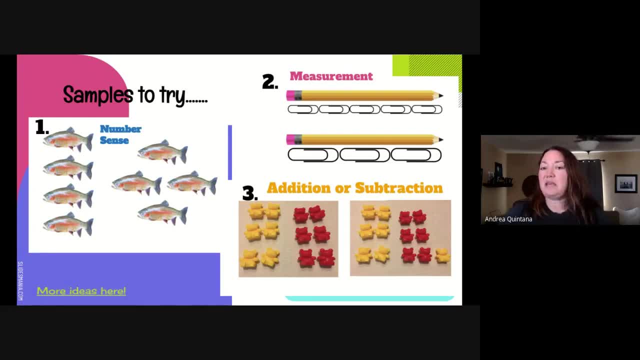 minutes of think time. How are these the same but different? And I'm looking at the pencils and the paper clips. So how are these the same but different? And remember that we're thinking of measurement. I'll give you a minute to think. 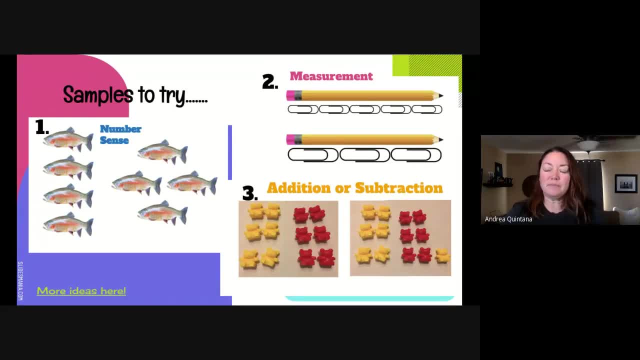 All right, hopefully you came up with one or two ideas about how these might be the same or different, And feel free to either type your answers into the chat and give me an idea of how these are the same but different, Or feel free to unmute yourselves, And I would love to hear you. 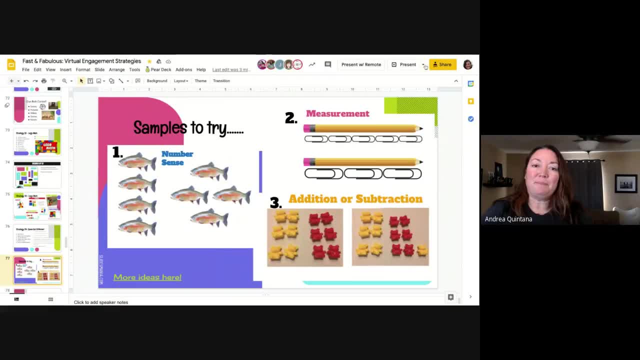 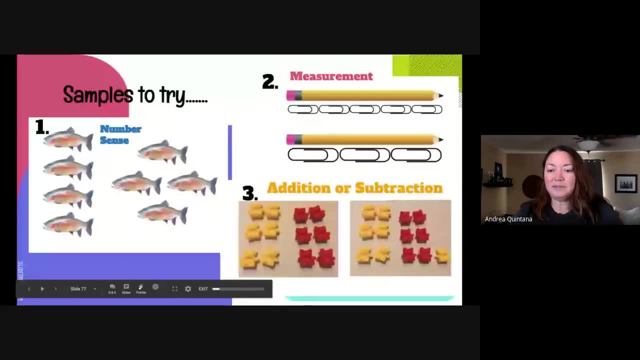 with your answers And I'm going to give you a minute to think. Words say how these are the same but different. Anyone brave today I can say what was in the chat button. but the pencils are the same length, but the units of measurement are different. Thank you, Tricia, That's perfect. What would? 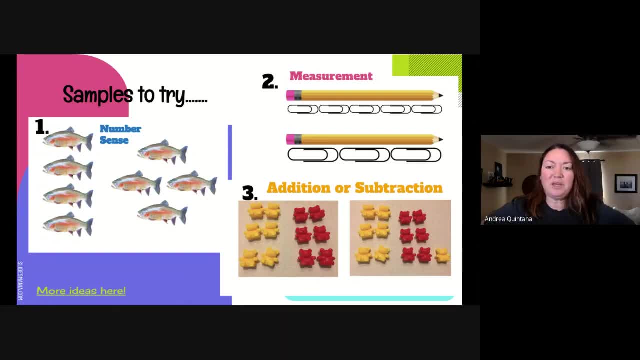 make the units of measurement different. Here we can find some more math vocabulary words as well. I can see that the smaller paper clips, I counted five, And the larger paper clips, I was able to only count three. And so by encouraging some talk, moves in with your. 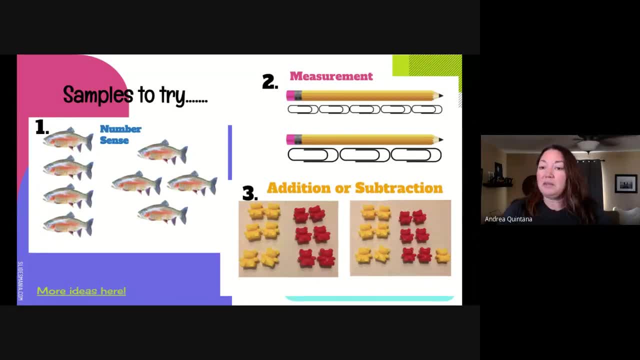 students. you're going to build in more of that math vocabulary and get them to really use some critical thinking to find ways that things are the same but still different, And so this was just a great idea, because students are very visual right now, but we want to make sure that we're. 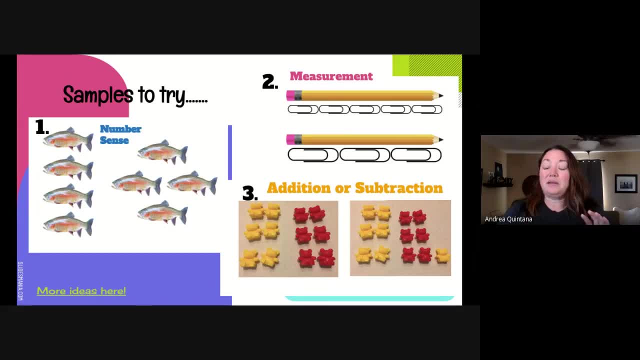 able to do that. We want to encourage some participation with them, And there are some great images out there that we could talk for days about. So let's use some math thinking and some math words to start some conversations. So this was a strategy that I thought might be fun. 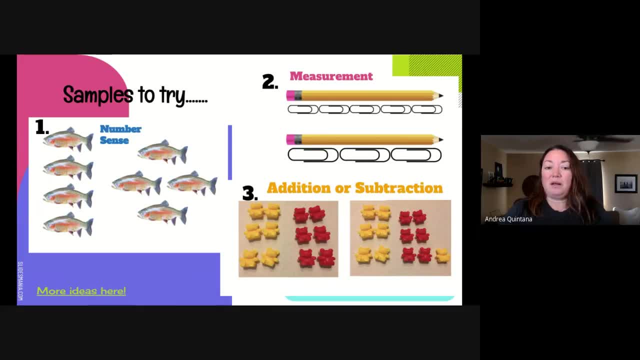 and really pull in some curiosity with your students as well. Again, that site is linked there for you: hundreds upon hundreds of images that you could share with your students. If you build it in with a routine and students start hearing those vocabulary, you're going to be able to. 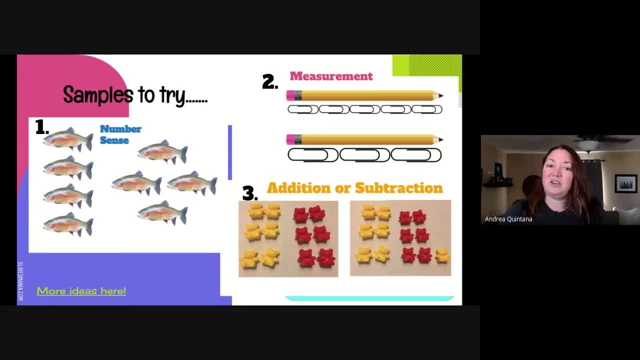 use it in a lot of different ways. So, if you're going to be able to use it in a lot of different ways, you're going to be able to use it in a lot of different ways. So, if you're going to be able to, 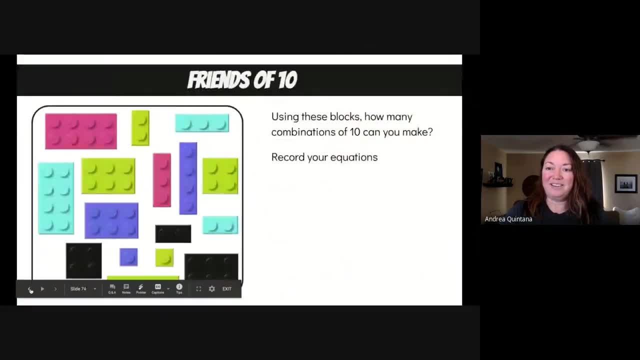 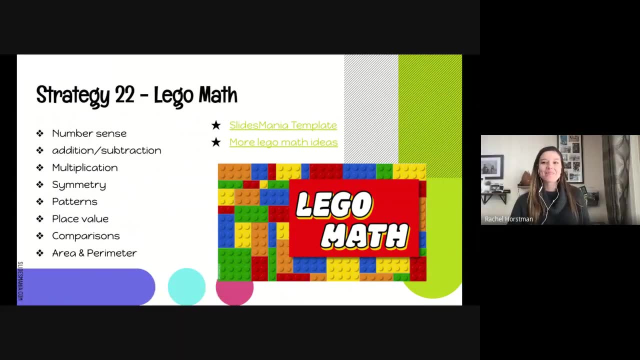 use it in a lot of different ways. you're going to be able to use it in a lot of different ways, So hopefully you enjoy this strategy. Rachel, are we ready? All right, let's see it. I found them. They were just a little bit out of order. Here we go. So, going back to Lego math. 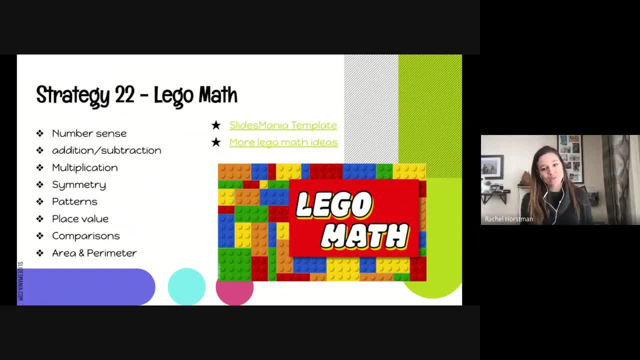 here's just a list, as I mentioned, of all the ideas you can use with Lego math. Going back to number sense, the strategy just Andrea just shared You can talk about. you know, if you're how to subitize your Legos right, Divide them up into different numbers and you've got your whole. 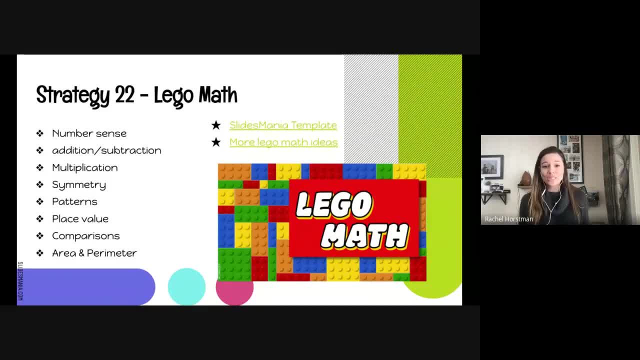 set there: Addition and subtraction, multiplication, symmetry, patterns, place value, doing comparisons which Legos have more dots and less, And then, like I said, area and perimeter. So these are clickable links here. Slides Mania is where I got this template from And, like I said, 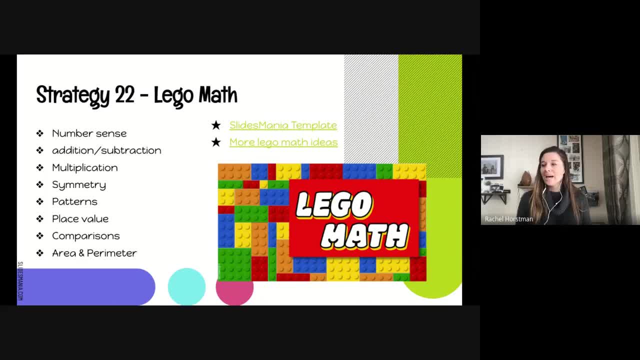 they already have some pre-made activities for you that you can edit. And then I found this great blog with just a ton of ideas to do with Legos in a physical classroom. But now, with the advantage of our Slides Mania template, you could easily make any of those activities. 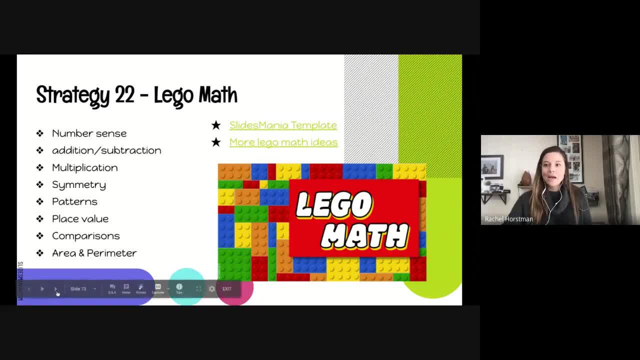 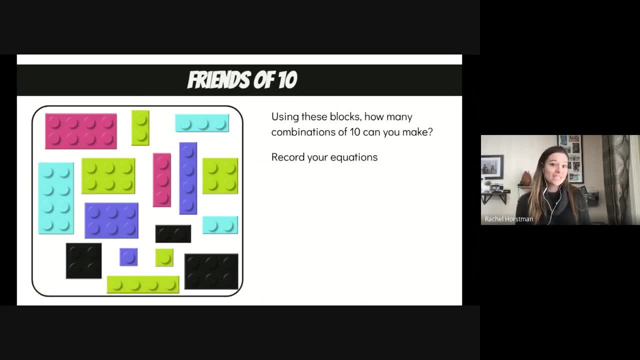 available for your students in distance learning as well. So this is the activity we're going to try. This would be great for our younger students thinking about friends of 10 or combinations to 10. We know that's an important skill for early number sense, So I've provided. 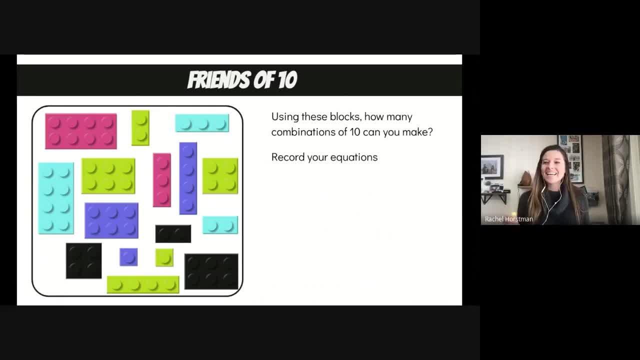 you know a set of Legos here And I would ask my students how many different combinations of 10 can you make And then record your equations? So if you gave your students editing access to this, they could move those Legos around and be physically counting. Or if you have some, 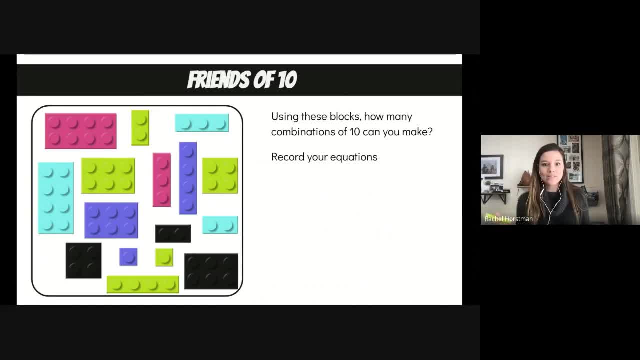 older students have them practice writing equations so that they have to make that connection. So I'm going to give you just about 10 seconds And you guys are going to record equations into the chat- all of the different ways that you can see 10 here. 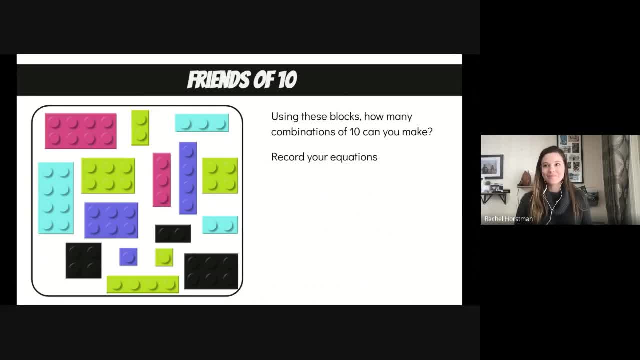 And feel free to press send as you have them. We won't wait on this one. I'm seeing 4 plus 3 plus 3, 6 plus 4, 8 plus 2, 2 plus 2 plus 2 plus 1 plus 3.. 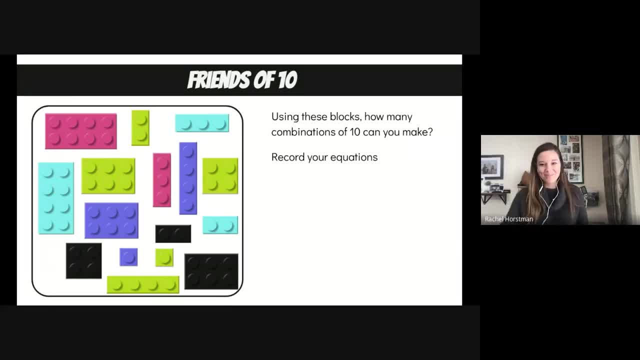 We're starting to come up with longer strings of numbers. That's great, Right, And then we can get into some deeper conversations again. So I might ask you know, Kathy, if she saw a different way, Or did she agree with somebody else's? Or I might ask her to. 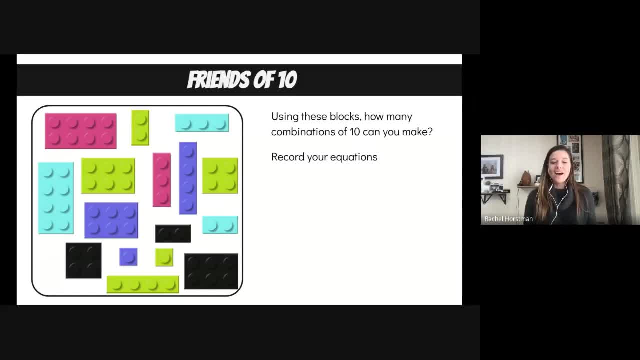 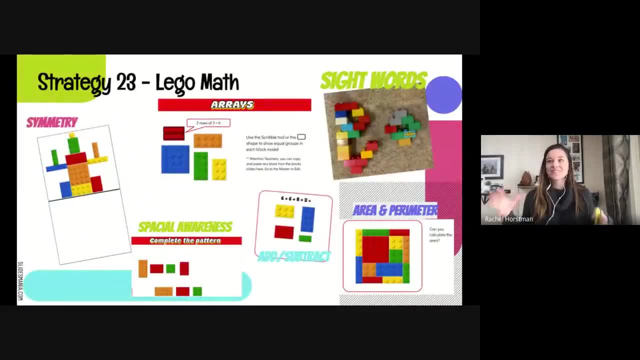 explain Andrea's thinking and her equation So that we can get into some more rich math conversations here And then, as I already showed you, here's just a whole bunch of different examples for how you might use Lego math in your classroom, And I hope that you find that useful. 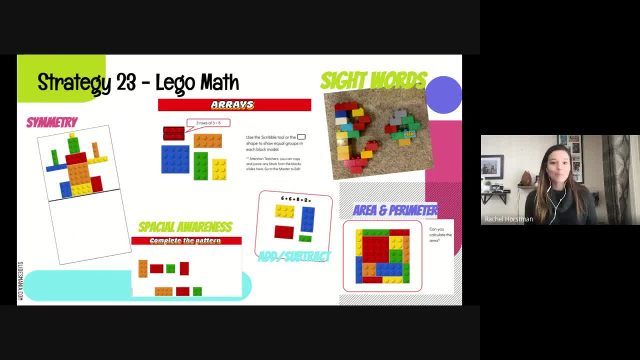 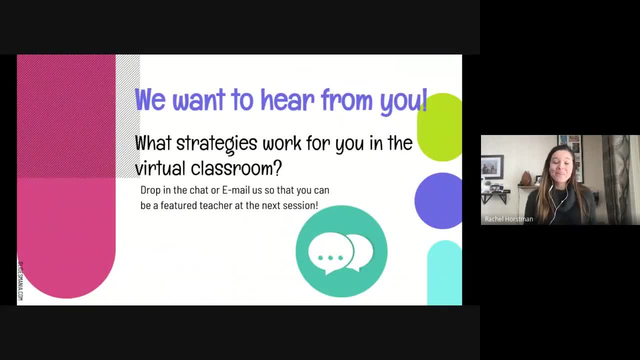 for your students to bring some hands-on materials that you might want to use in your classroom, And if you have any fun math strategies- I saw Jennifer already shared a website with us in the chat. We'd love to hear from you What's working well in your classroom already. 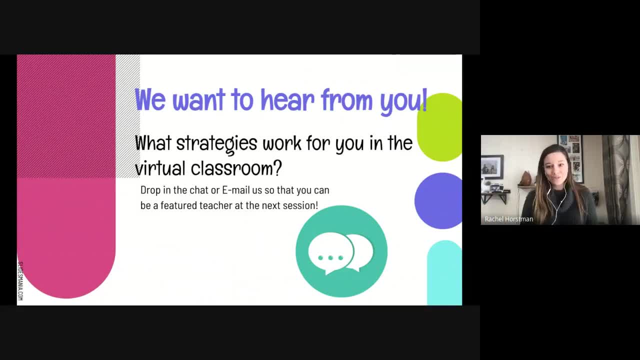 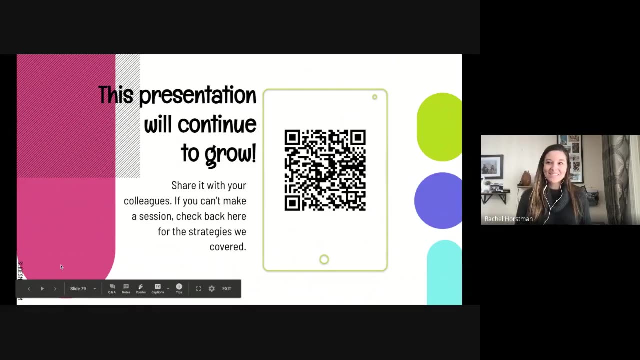 A lot of the strategies we share here we've learned from teachers like you, So if you have a moment, drop it in the chat. What is going well in math for you? And, as we also mentioned, this presentation continues to grow. We have more dates coming up. 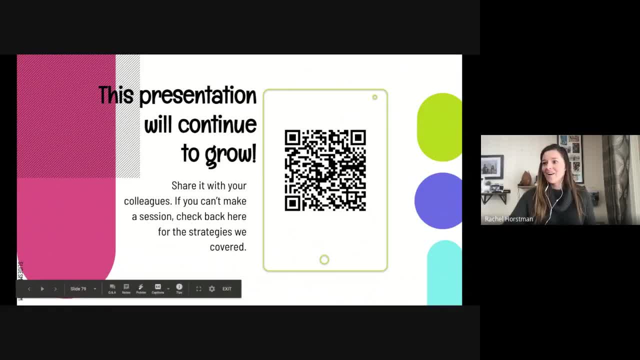 I believe we have another session this week on Kathy. do you remember what time? On the 9th. Thank you, Andrea. So next week we will have our next Fast and Fabulous- Look for that in our TLF chats- And we'll be sending out the flyer again, As always.